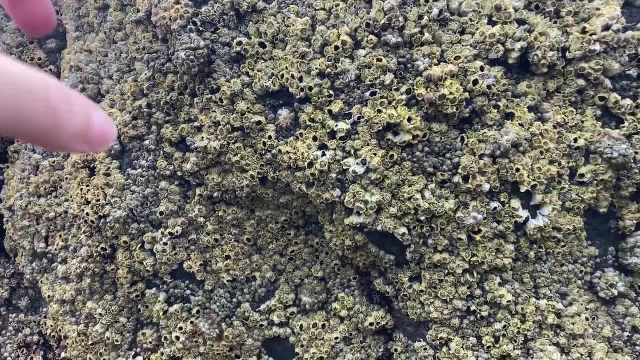 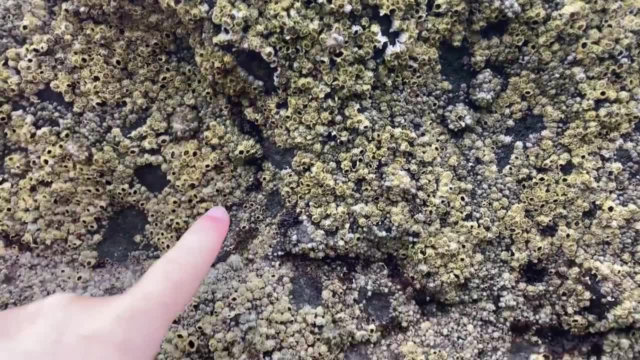 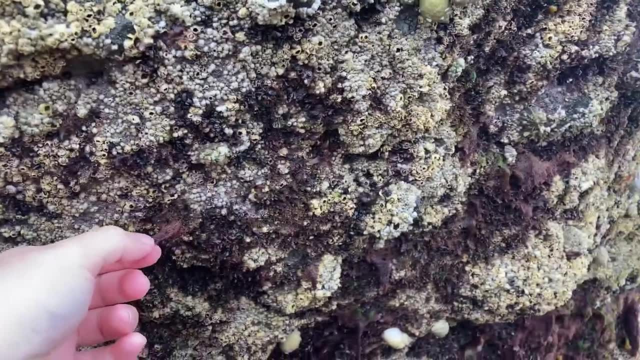 can't get these off. they're so tightly attached that they are keeping themselves attached to the rock so that no water escapes their body and they can survive. but as we start to move down and a bit further, we start to notice these patches. now this is seaweed starting to grow. 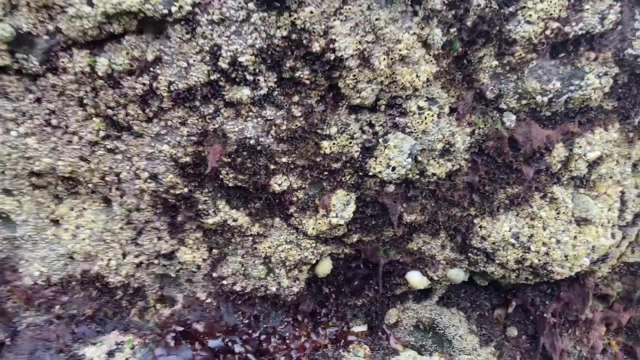 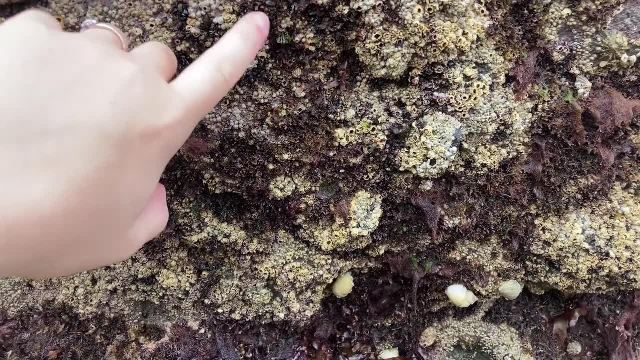 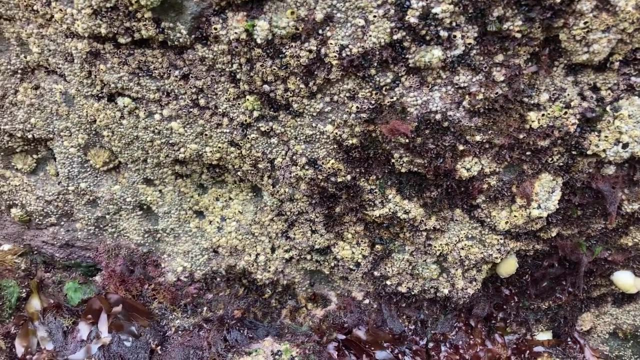 seaweeds are very different. each type of seaweed has different adaptations. so at the start we get some species that are adapted to surviving out of water, like this teeny, weeny little seaweeds here, um, but as we go further down, we start to introduce new species. now what really? 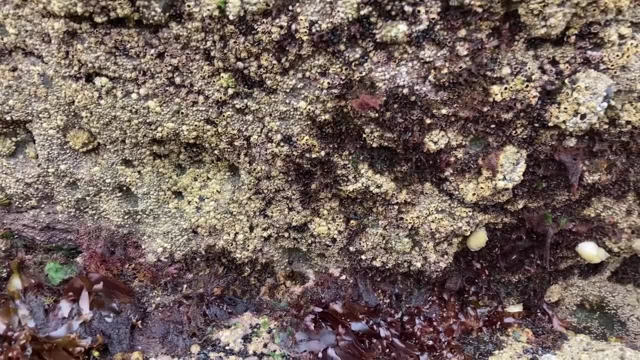 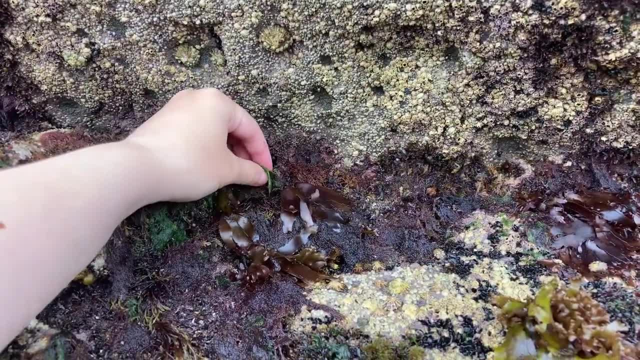 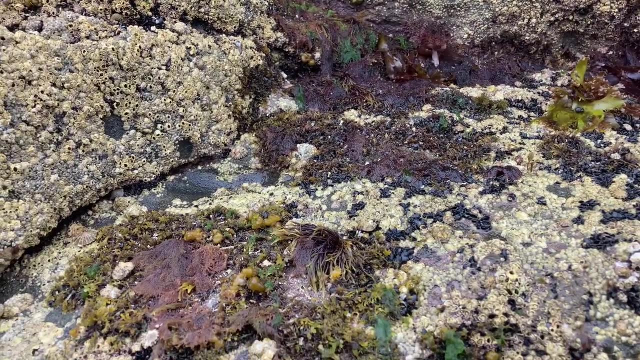 can't stand. um. drying out is often a lot of species that are red seaweeds, and so you won't find so many red seaweeds. you'll find browns, and potentially you will then start to find green seaweeds as well. as we move, started down, we'll start to see more and more color. this is more. 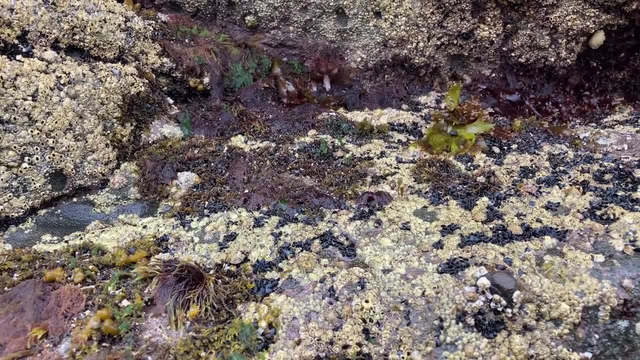 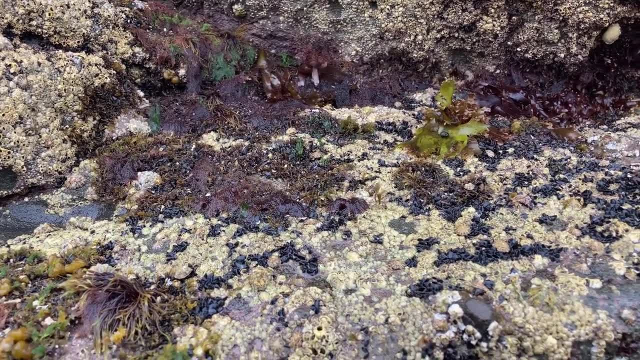 and more seaweeds being able to live in a zone where um there's enough water for them to live. they're not having to adapt as much to living outside of water, and so more species can find a home. but as we get further down, more and more competition happens because more species 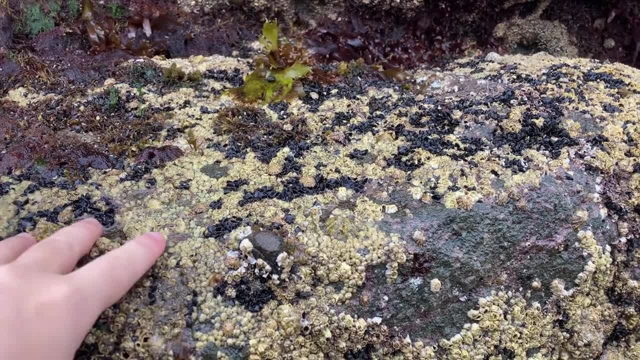 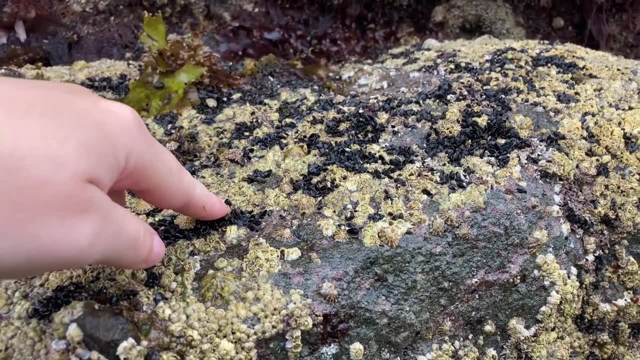 are able to live there, and so more species are fighting for the real estate of the rock. we then start to hit things like mussels. now, mussels can close up, which means they can survive out of water for a long time, but they're not as well adapted as some of the other species. 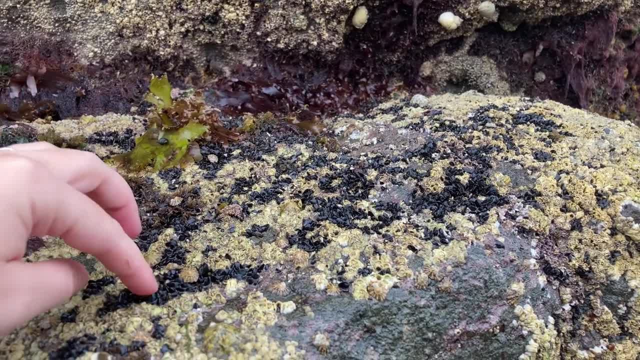 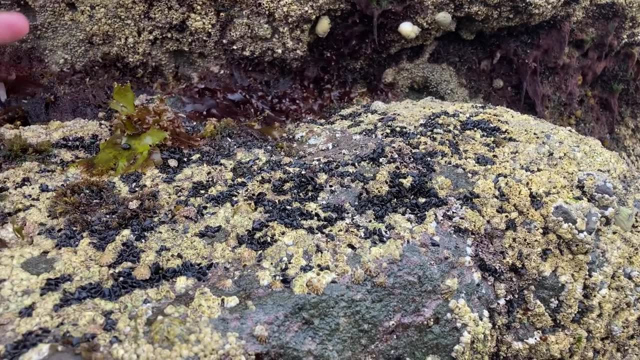 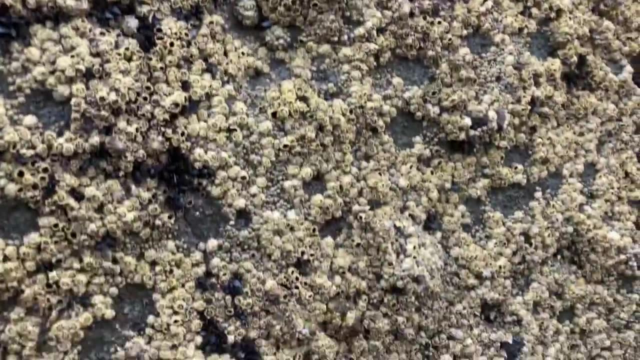 so they're not found at higher up. this is also a species of muscle called modiolis. you won't find um bigger muscles. sometimes you won't find them higher up on the shore because they need a lot more time in water to survive. now we start to work our way right down. 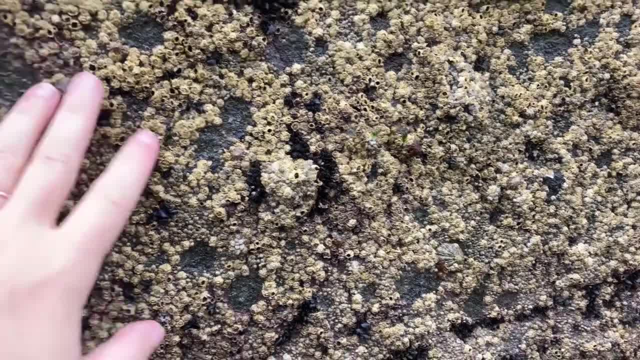 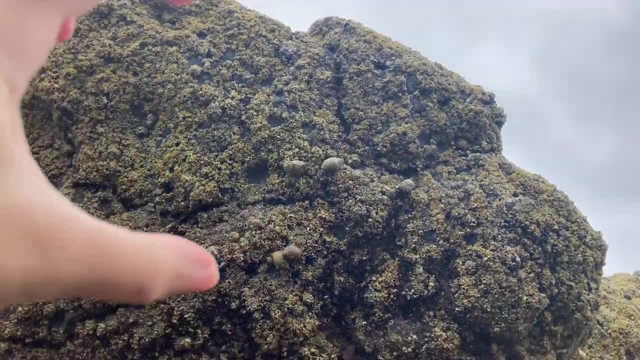 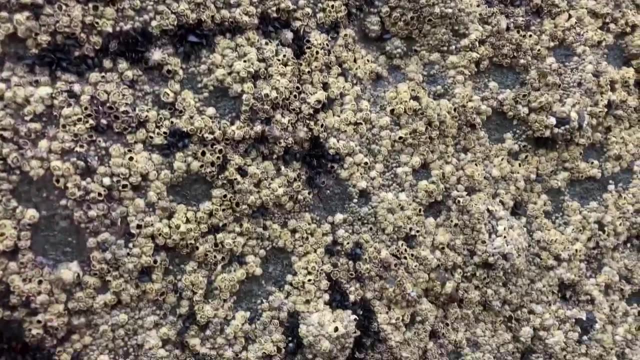 the wall and you may notice that a lot of this is the same. it's not so different. you've got, you've got the top zone which is about that big and that's just a species really really adapted for the shore, and then you've got this, which is all really the same. now you can 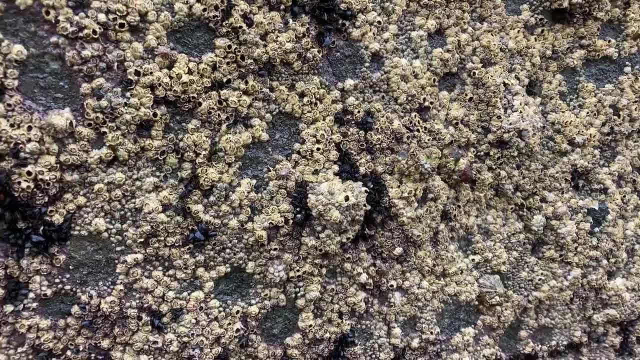 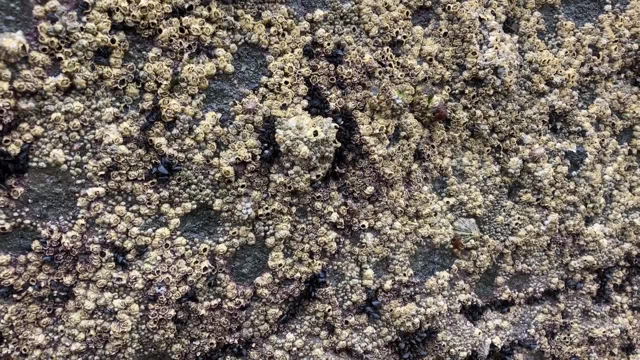 call this midshore. this is the midshore where species are in this water. for a bit they're out of water for a bit there's adaptations needed. but you still can't live here if you're not adapted very well to live out of water. but you'll notice a really 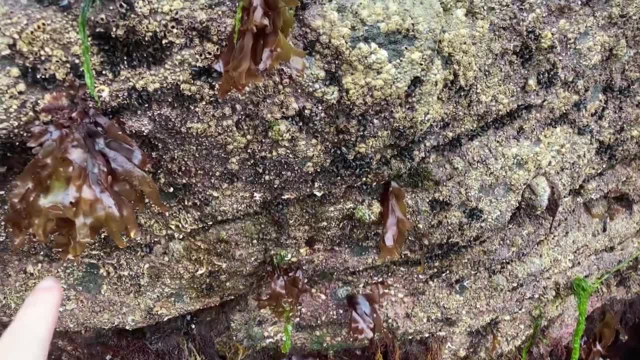 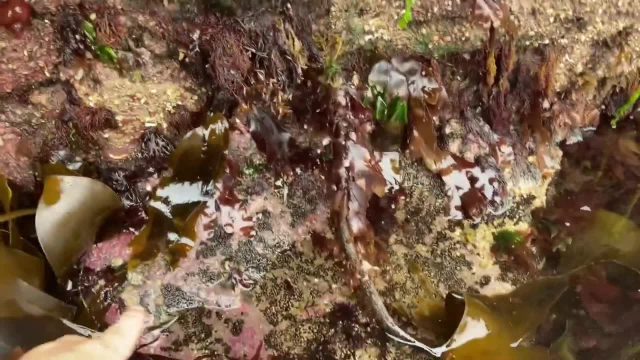 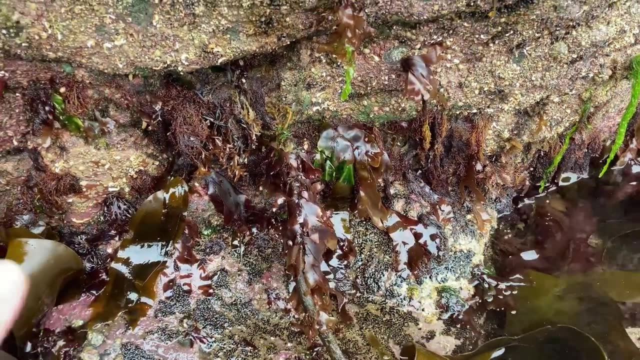 stark change all of a sudden here now- this is what you can call low tide- we start to get some of the red seaweeds that i was talking about. this stuff here, this pink stuff, is crusto's algae. this is an algae that grows along the surface and forms a calcium carbonate skeleton. 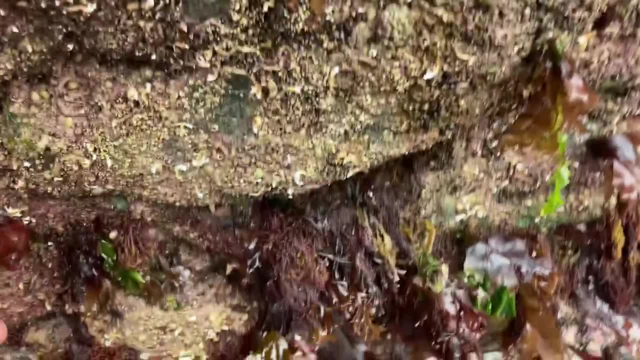 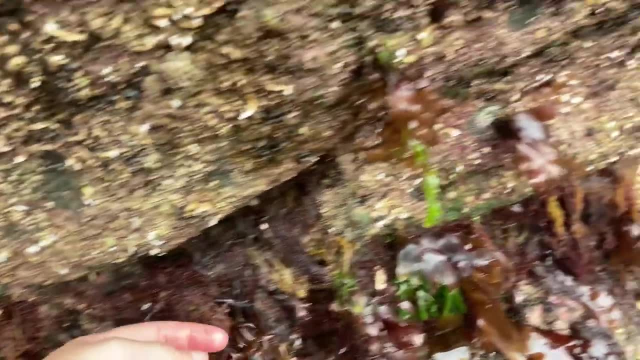 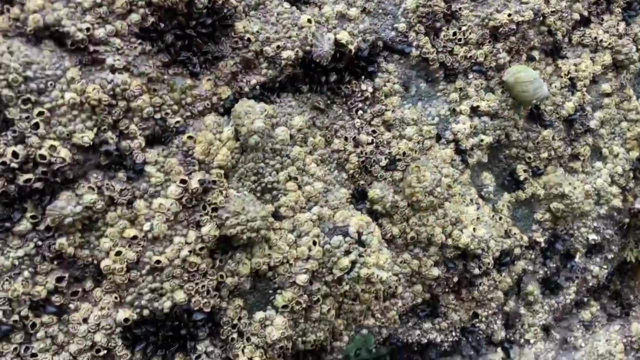 a bit like coral. we also start to get some fabulous animals here. this is a an anemone loads of different, more green seaweeds. this is a red seaweed called bunny ears, and this is another red seaweed, green seaweeds, limpets- you've got lots of snails. this. 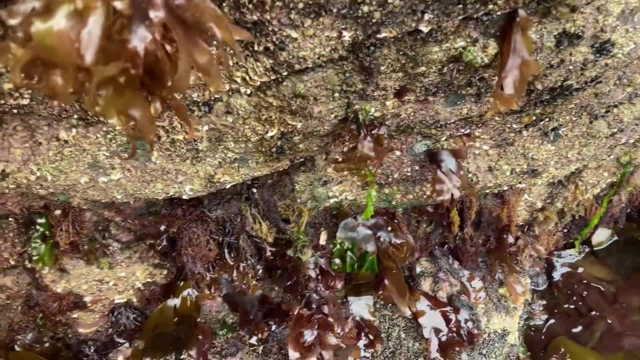 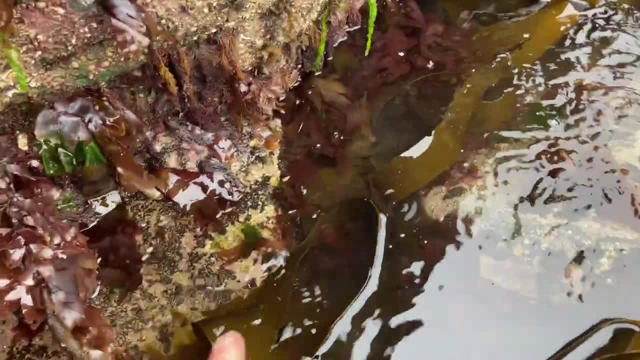 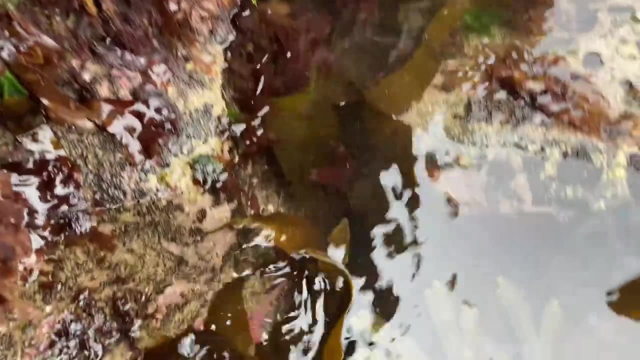 is a much more productive zone and lots more species that live here, because the water is literally here. it's only out of water for maybe an hour every day, and this here is kelp, and this is always found at the lowest of the low shore. it marks the boundary, really. 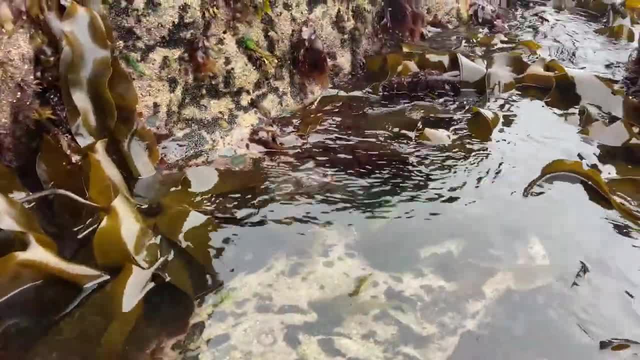 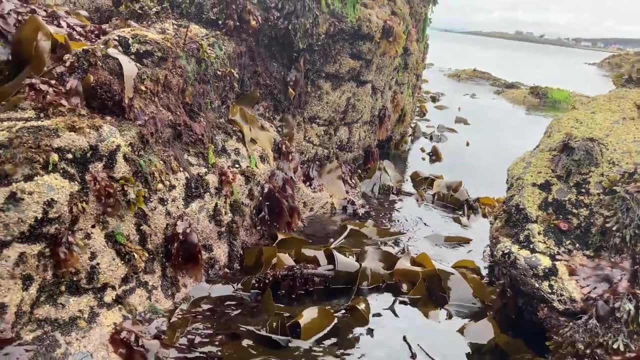 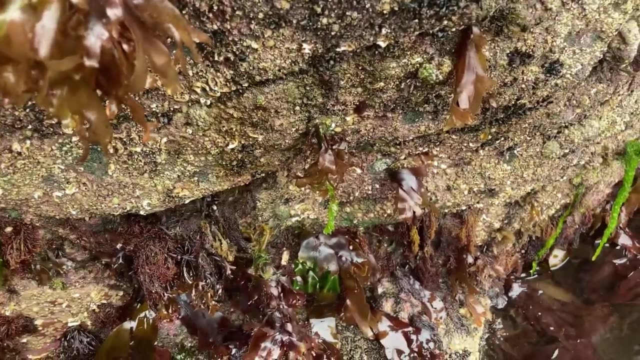 between an intertidal zone and a subtidal zone, so a zone will always stay in the water and you can tell that by the kelp beds that start to form at the bottom. but what's interesting about this zone? there will be a lot more species, but it will be a lot more competition. there isn't many gaps in. 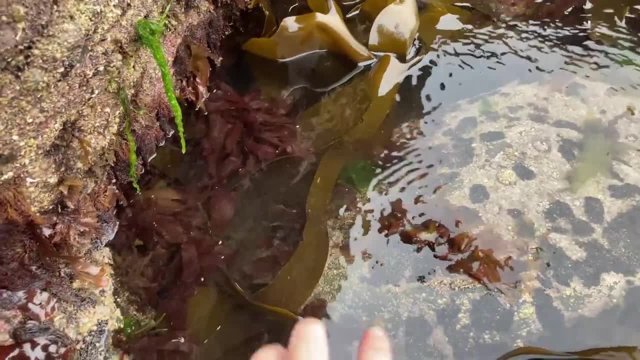 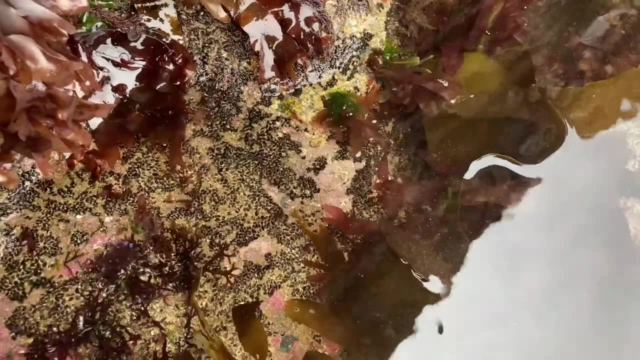 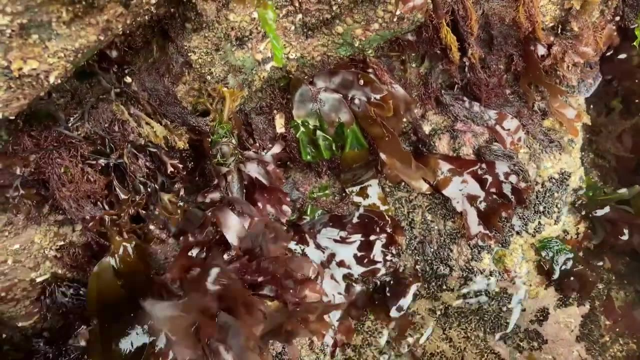 the rock. here, where there are gaps, it's because limpets have been feeding and there's a lot of stuff going on here within. you know, within the space of a few um, we've got sponges, crusto's, coral and algae. this is condus crispus. we've got a type of muscle. we've got another species. 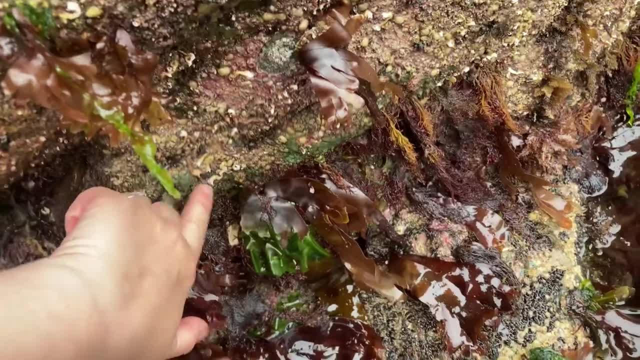 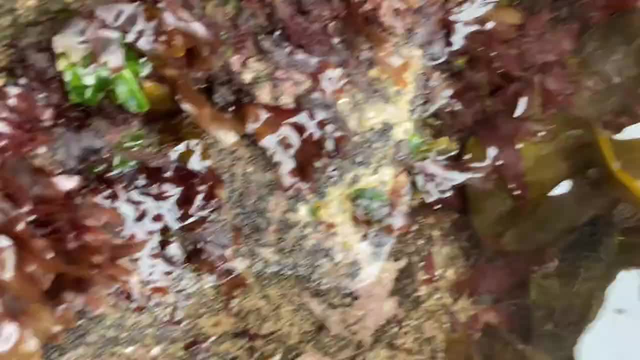 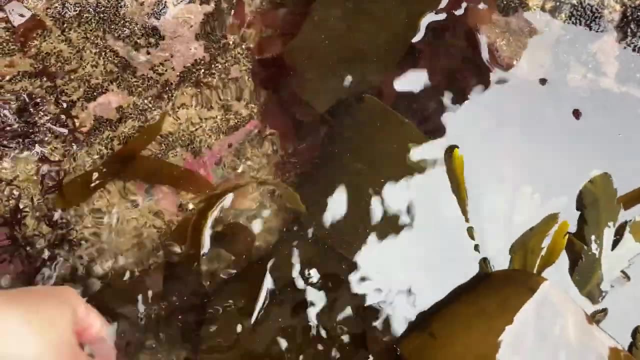 of algae. we've got kelp. we've got tube worms. um, we've got sea lettuce. we've got an anemone. uh, what else have we got? we've got bryozoans growing on this piece here, limpets. this is a type of fucus seaweed which can live here. this is another type of red seaweed, another anemone.